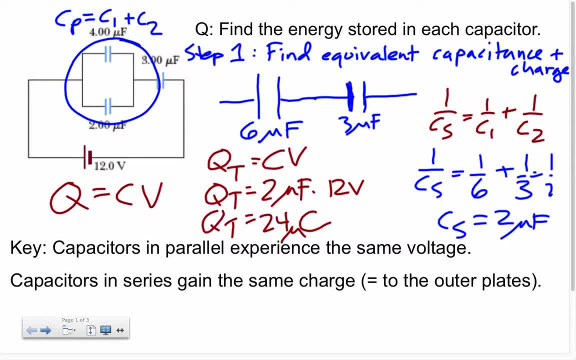 Where is that charge? Well, if you got capacitors in series, right, that charge had to come from the other capacitor because there's like a gap in each capacitor. So there's 24 here and then there's 24 over here. 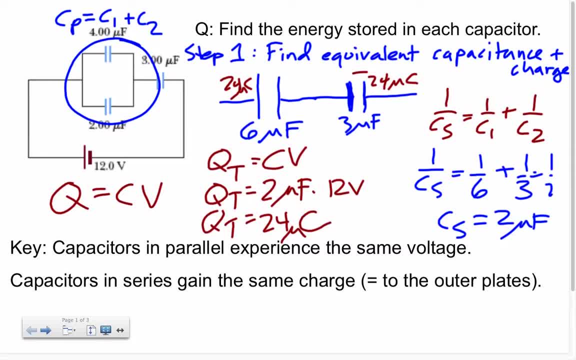 This would be negative in this case, right? And so there's like positive 24 on this plate, negative 24 on that plate, and that charge had to go from one plate to the other. That's why it has to be the same everywhere. 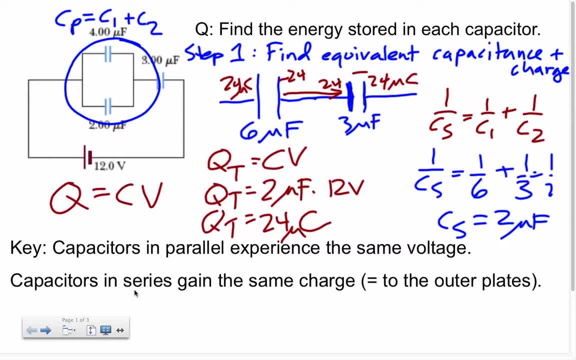 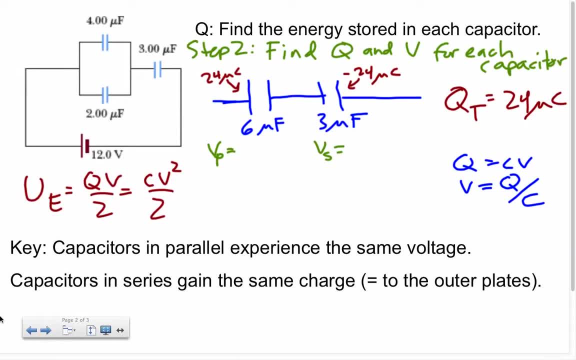 So now that we know there's 24 on each plate, we can actually start to figure out the rest of this problem. So we know there's 24 here, 24 there. Now the step is to find how much potential is you know across each capacitor. 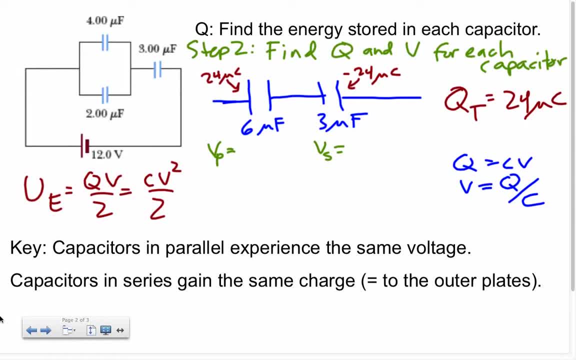 What's the difference of potential for each one? Well, we can just use this handy dandy thing, right, Just simple relationship. So we got 24 over six, 24 over three, The potential across the parallel, which is the same for both. right, got these key little. 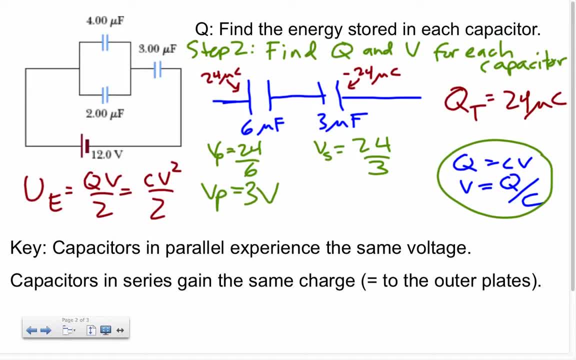 things to remember. on the bottom, here is three volts, Wait 24, four volts, And for here it's eight volts. Oh hey, those add up to 12.. That makes sense. So now we know how much potential is across each one. 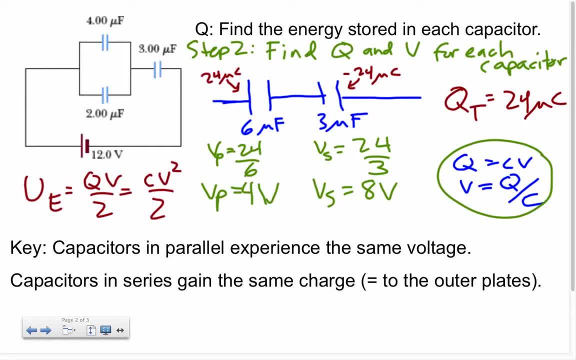 Well, wasn't this four volts across six? I guess that means you have each of these two in parallel. There's like a four-volt difference across each of those two, right? If we make a picture of the circuit, you might be able to see this a little bit better. if. 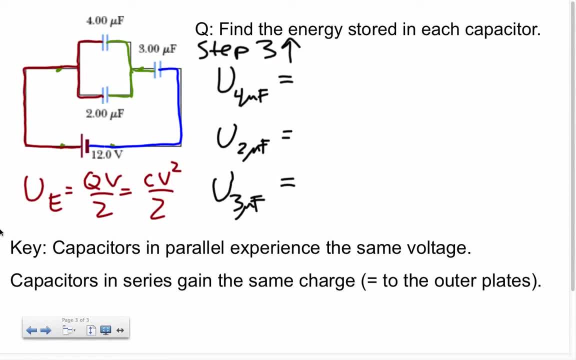 we color code things. So this is the last step. right Now we can finally determine the energy. There's basically a high potential all along here. on the left side There's 12 volts. right, if we say zero is the negative plate. 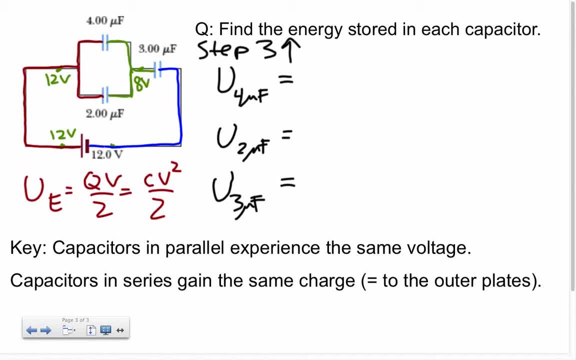 And then it drops four volts to eight volts here, And then on the right side you're back to zero volts right, And there's a difference across the gap of each capacitor, And the two parallel ones share that difference of four volts.